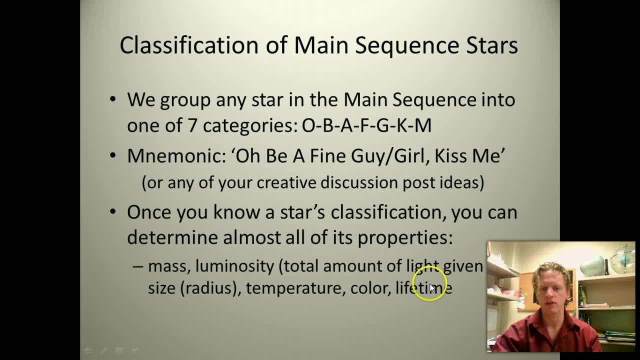 density, or its size or its temperature or its color or its lifetime. we can know every other property of that star as long as it's a main sequence star, as long as it falls into one of these seven categories. So if I were to tell you that we're dealing with an O star all of a sudden, you would 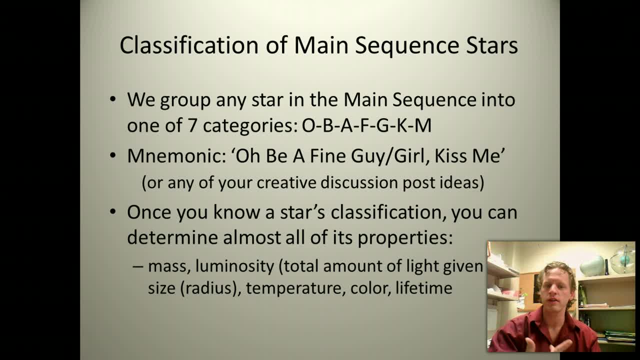 know all of those properties. You would know roughly what its mass is, you would know its luminosity and blah, blah, blah. If I tell you that our sun is a G-type star or if you have one other G-type star, if you 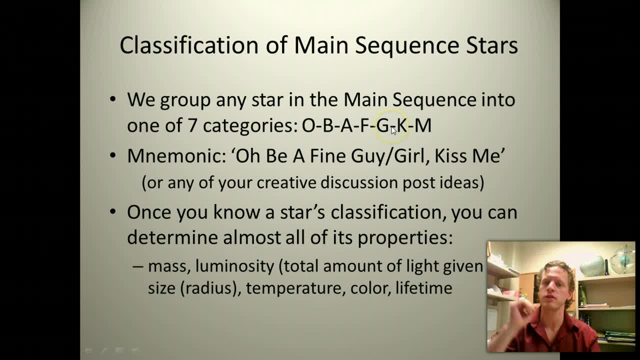 know some other star is a G-type star. you'll know it's very similar to our sun, which is a G-type star, And so if you know our sun's luminosity, if you know our sun's mass and if you know our 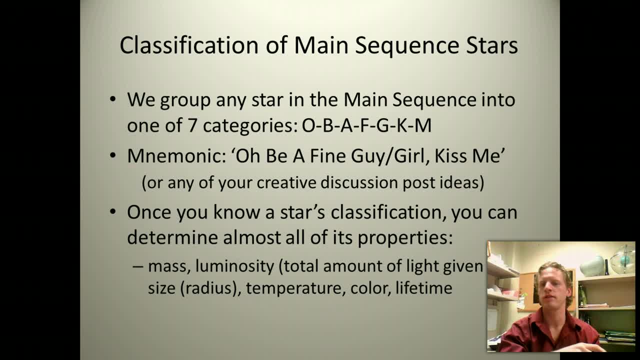 sun's temperature, for example, you'll be able to roughly guess at the mass, the temperature, the luminosity of this other star, because it's the same class of star. Now, obviously, not all G stars have exactly the same numbers and not all M stars have. 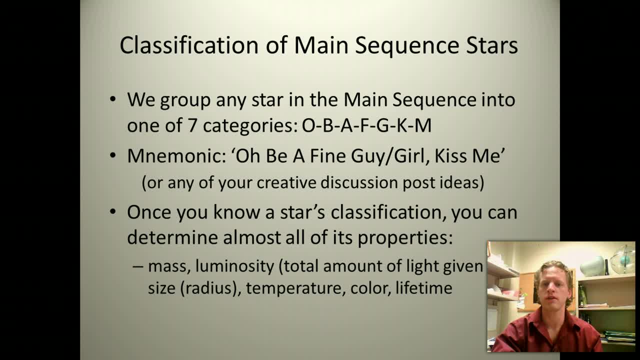 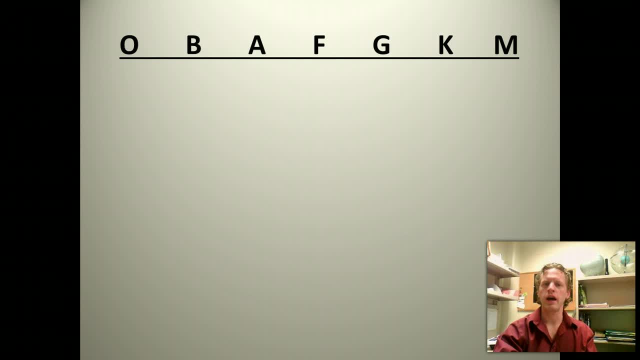 exactly the same numbers, But to within 10% or so, all the stars in a single class are roughly the same, So that's why this is so important. So just going through each of the properties and how: mass luminosity, color temperature. 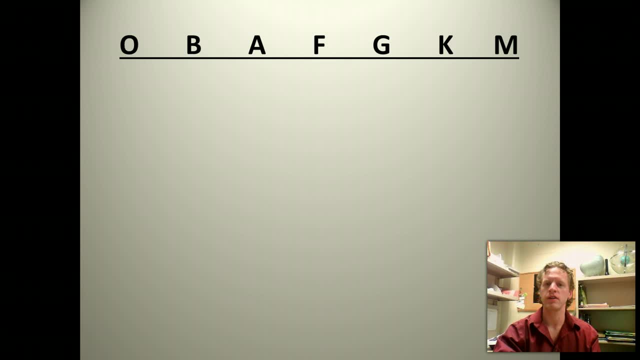 radius, lifetime, How all of those things are related to its classification. So first of all, mass. The most massive stars are the O and then the B-type stars. These stars have the very most mass going on the other end, the G and then the K and 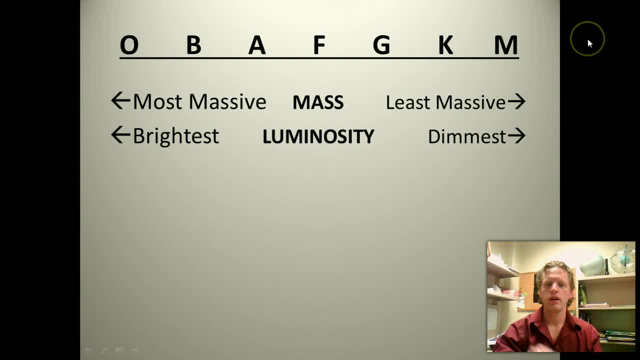 then finally, the M stars are the least massive stars- The luminosity- So, by the way, luminosity is just a big word for how much total light the star gives off. The brightness, essentially Not necessarily how bright it looks to us- we'll get to that- but the total amount of 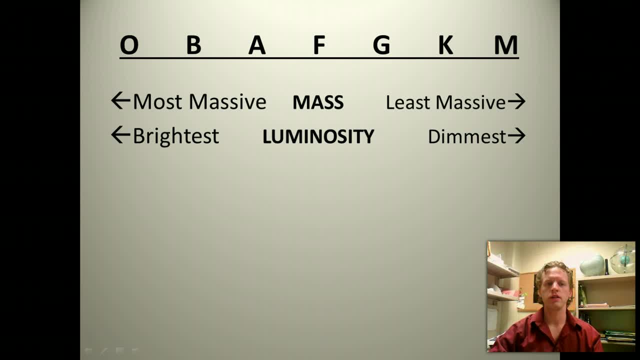 brightness that the entire star is giving off, And it turns out the most massive stars are also the most luminous. The stars with the most mass, the O and then the B-type, also give off the most light, And I think that kind of makes sense conceptually. 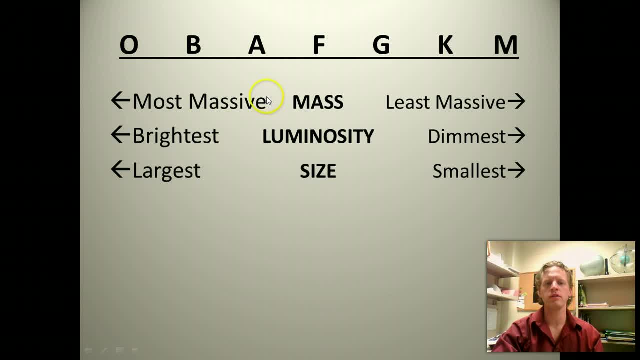 Next is the size, And this is again kind of obvious. If you have a very massive star, the most massive stars are also the very largest. So you pack more mass into a bigger star. the smaller the star gets, the less massive it gets. 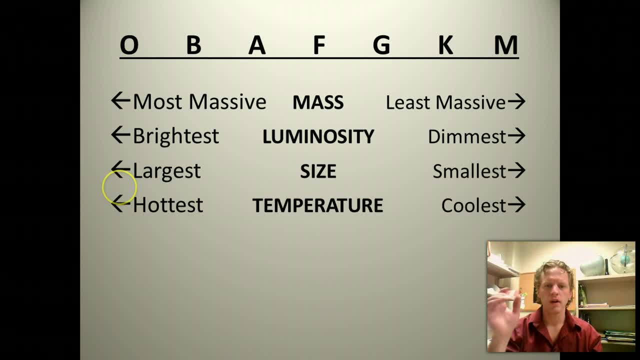 And again common sense, but that's how it works. The temperature And just like these other things, The stars- the most massive, the brightest, the biggest stars- are also the hottest stars. So O-type stars are incredibly hot: over 30,000 Kelvin. For example, our sun is only about 5,800 Kelvin And M-type stars are. they can be around 3,000 degrees Kelvin, So it ranges all the way from 3,000 Kelvin to over 30,000 Kelvin. 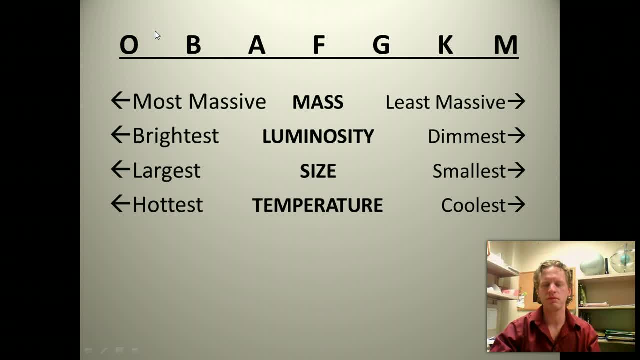 By the way, you can roughly double that and that's about the temperature Fahrenheit. it's not an exact number. Okay, the color It turns out. all M-stars have roughly the same color and they're mostly red. orange is red. 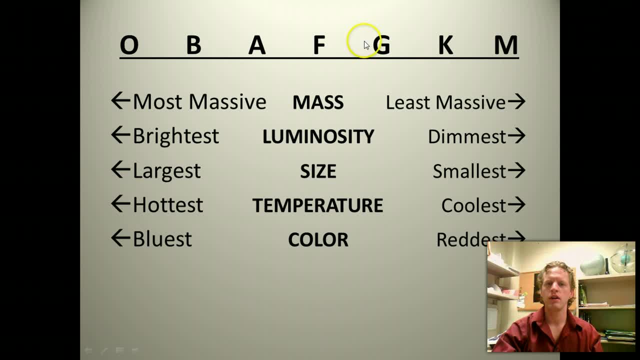 As we go from red stars here it gets a little more into the yellow range and greenish, and then bluish, violet or even ultraviolet. So O-stars and then B-stars tend to look blue to our naked eye actually. 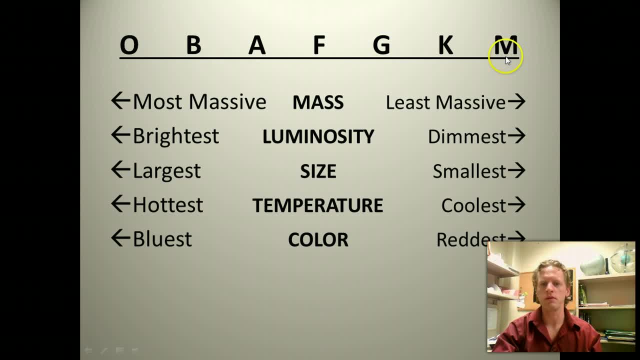 You can actually see some of the bluer stars out there, And then K and M-stars very much look red to our eye. One of the examples of a red star would be B-star. Okay, Okay. So this is a star called Betelgeuse, if any of you are familiar with them. 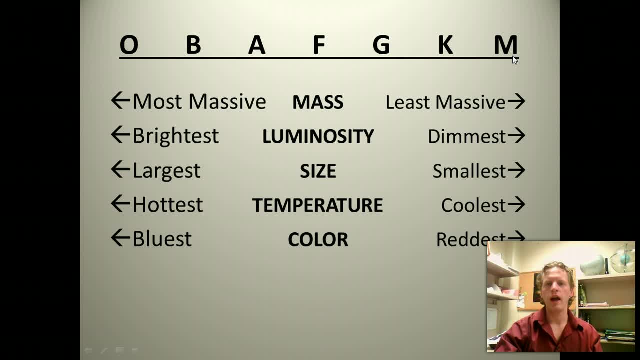 It's one of the stars in Orion. It actually looks. it has a reddish tint, And just above Betelgeuse is Rigel, known among other things from Simpsons fame. It's where Kang and Kodos are from Rigel 7.. 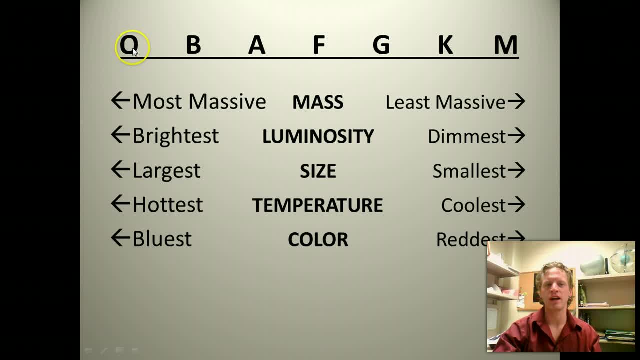 Anyway, Rigel, which is also in the constellation of Orion, looks kind of bluish to the naked eye and it's an O-type star. So the color: if you look at its color, you can tell what type of star it is. And finally, the lifetime. Now, this is counterintuitive. We will get to this a little bit, But it turns out the very longest-lived stars, the stars that live the longest, are the M-type stars And the very least massive, I'm sorry, the very most massive stars, the O-type stars. 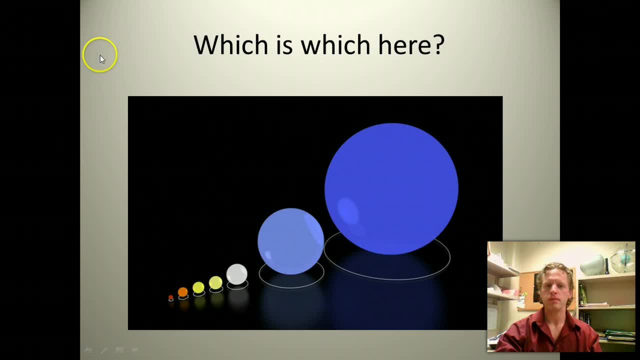 have the shortest lifetimes. There's a reason for that, but we'll get to that. So just to kind of sum it up, which one of these stars is which class? I'll let you figure it out. I mean, I guess it would have been more complicated if I put them out of order. but yeah, which? 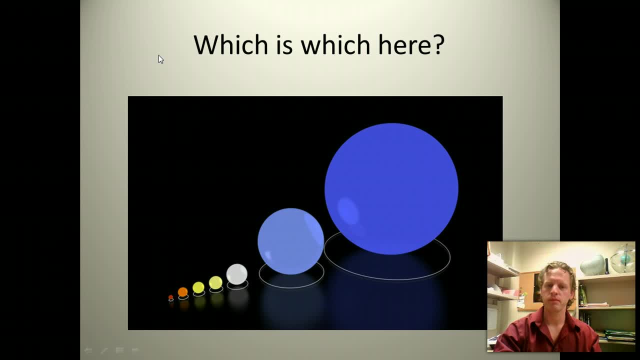 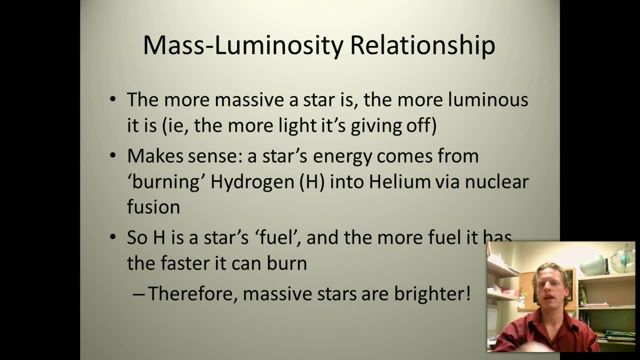 one are O-type stars, which one are M-type stars and which ones are in between. So, okay, I want to go through a couple of the relationships: How is mass related to luminosity, How is color related to temperature, How is lifetime related to mass, and so on? 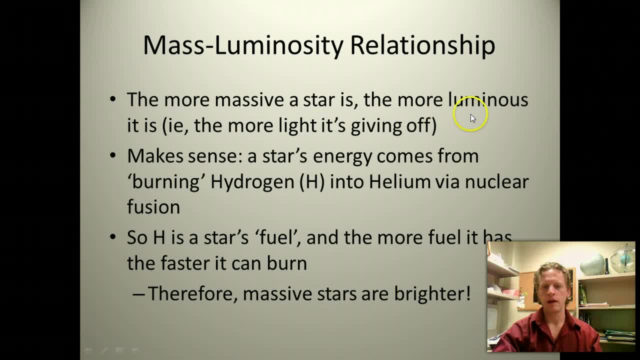 So the most massive stars, like I said, are the most luminous. That means the more massive a star is, the more stuff it has in it, the more light it's giving off And conceptually the way this makes sense to me is that basically the light from that. 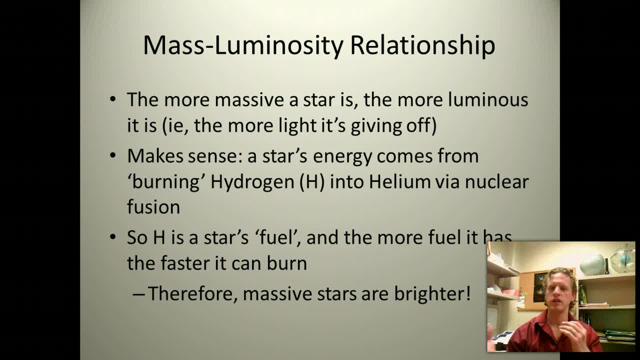 star comes from nuclear fusion. When you're taking hydrogen and turning it into helium, it gives off light. So the more hydrogen you have, The more light you can produce, because basically you're burning through your fuel. The more fuel you have- which in this case the fuel is the hydrogen gas- the more fuel. 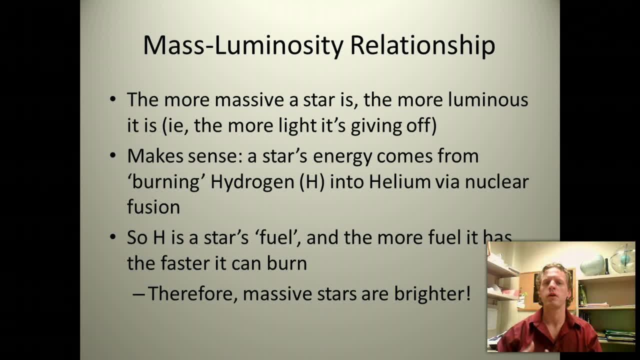 you have, the longer you can burn your. I'm sorry, not the longer, but the more fuel you have, the more light you can give off. And that's what's happening. The most massive stars have way more fuel, so they're giving off way more light. 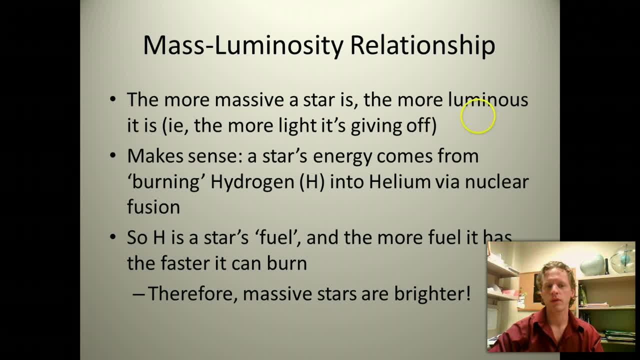 They're burning through that fuel because they have a lot higher store of it to begin with. So the most massive stars give off the most light. That means they're the most luminous. When there's an exact relationship, it turns out that the luminosity goes as mass to the 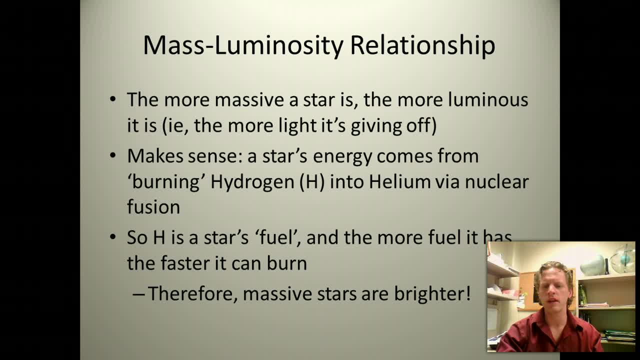 3.5th power, if I'm correct. You don't need to know that. It mentions that in the lab for this week, but you're not going to need to calculate exact figures, But just understand that luminosity rises as the mass rises. 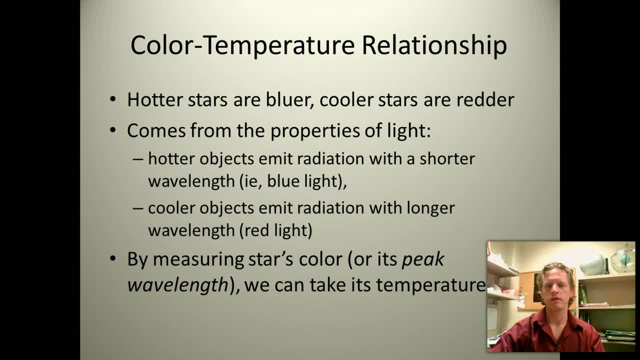 Okay now, how is the color related to the temperature of a star? So, like I said, the very hottest stars were the most massive and the very bluest stars were also the most massive. I guess it would be that direction for you guys. 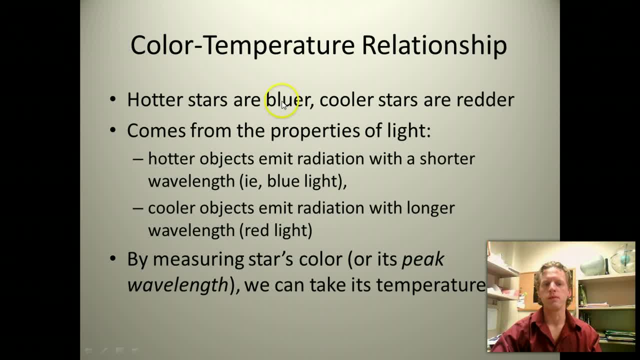 But anyway. so the very hottest stars are blue and the very coolest stars are red, Turns out that's actually a fundamental principle of how light works. Any object that's very hot gives off very blue radiation, And actually it turns out that the hotter you make something, so you might start with. 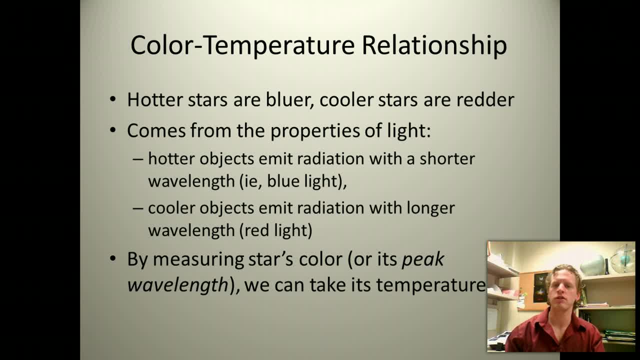 something that's cool. that's maybe giving off reddish light. You increase its temperature so you might go from red to kind of orangish light that's giving off to maybe yellow, And then you increase the temperature even more. it starts giving off blue light. 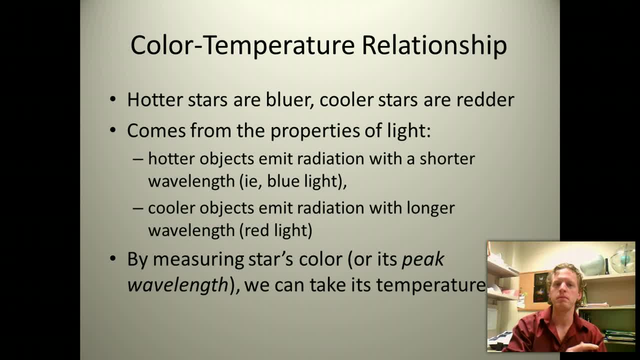 If you keep increasing that, it will actually turn to ultraviolet. Ultraviolet light is giving off And some of the most massive stars out there, some of the very hottest stars, are giving off, mostly ultraviolet light. Now, on the other end of the spectrum, the very coolest stars are the ones that are giving. 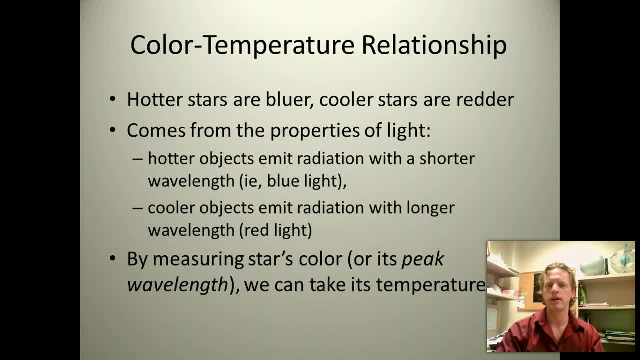 off mostly red light, And if you've ever sat around a campfire, you actually know this, because if you have a very hot fire, all the ashes are incredibly hot. most of the ashes are white or most of the burnt logs are glowing bright white, which is a combination of all blue and orange. 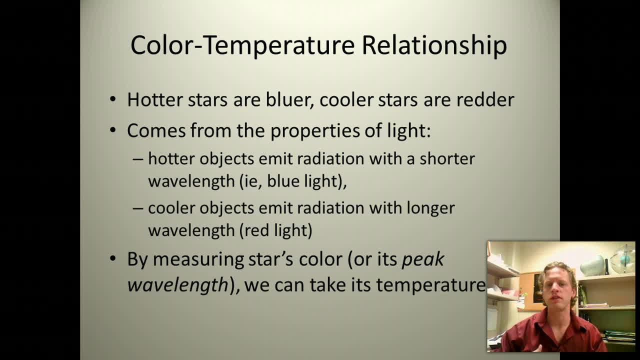 and yellow and red and everything. And if you have a really cool fire, once it's died off, once it's almost dead, those ashes turn just kind of a dullish red color And you can actually tell the temperature based on how much red light or how much blue. 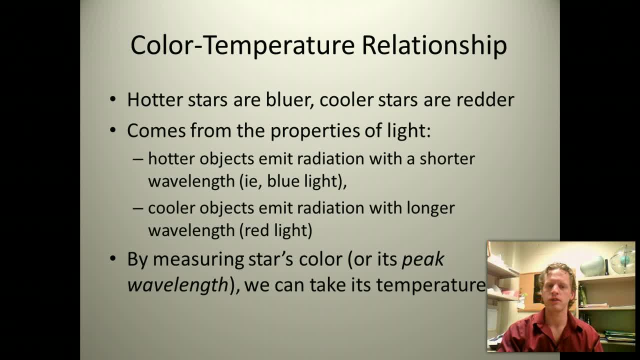 or those other types of light on the blue side of the spectrum it's giving off. So again, the point is: the redder something looks, the cooler it is, and the bluer something looks, the hotter it is. And the nice thing is we can actually directly measure the temperature on the surface of 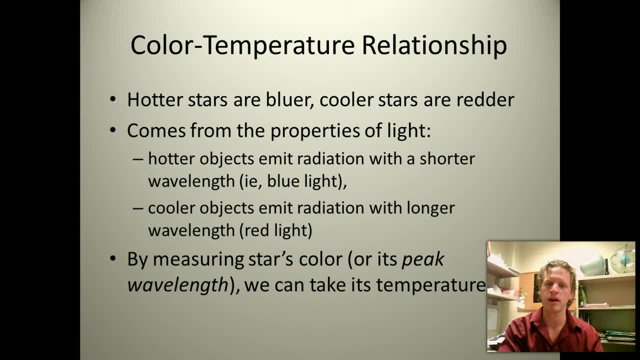 stars that are thousands of light years away, just by looking at what type of light they give off. Is it blue or is it red, or is it somewhere in between? There are exact ways of measuring exactly the temperature, but we're not going to get. 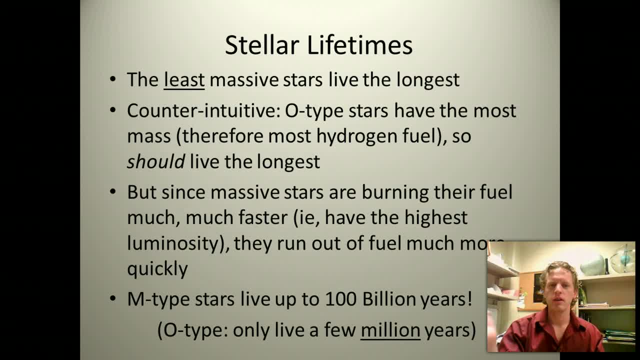 into that in this class here, or at least not yet. Okay, so the other one that I wanted to mention, because this is a little bit counterintuitive, and when I learned this it didn't make sense to me either, but it turns out that the very 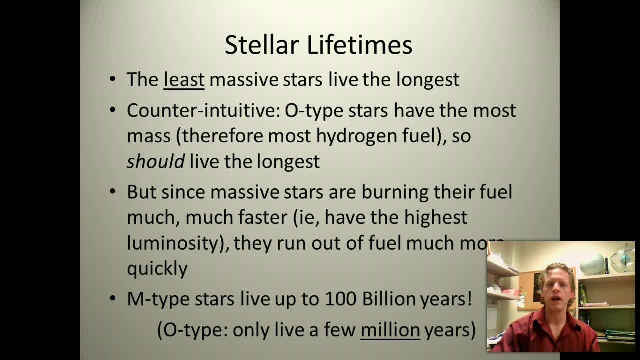 least massive stars have the longest lifetimes. So those M-type stars live way longer than the gigantic, extremely massive O-type stars. Now the reason for this actually makes sense once we think about it: The most massive stars have way more fuel, Way more hydrogen gas to burn. 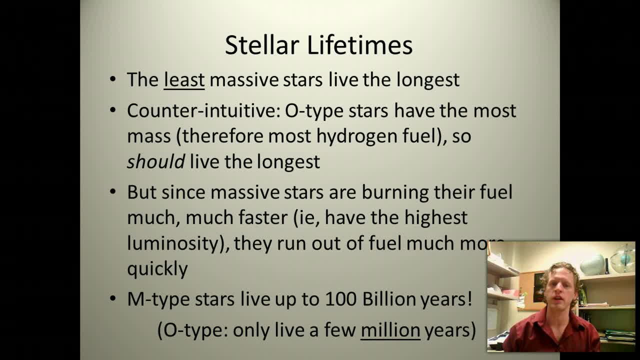 But they're also the very most luminous Way, way more luminous than the other types of stars. So that means that they're burning through their fuel way faster than the M-type stars or than the K-type or the G-type stars. 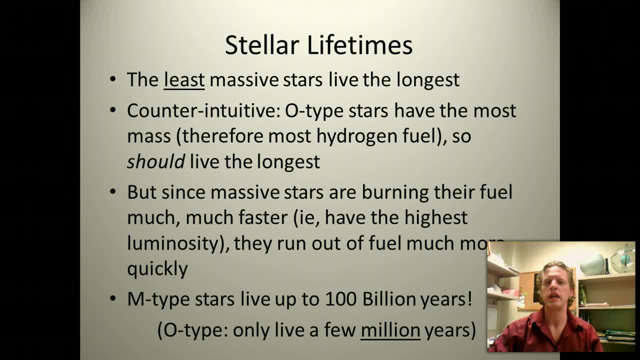 And the faster you burn through your fuel, the faster you're going to run out of it. So, even though they start with more fuel, they're burning it way, way faster than those low-mass stars that don't have much luminosity. 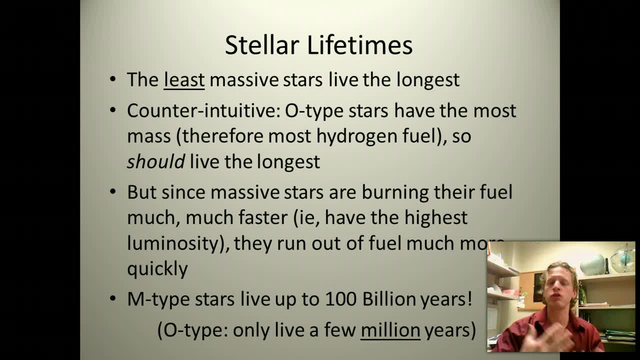 So it turns out that the more mass you have, the faster you burn through your fuel and the shorter your lifetime is in fact Now the O-type stars, I'm sorry, the M-type stars, these very low-mass stars, their luminosity is very low. 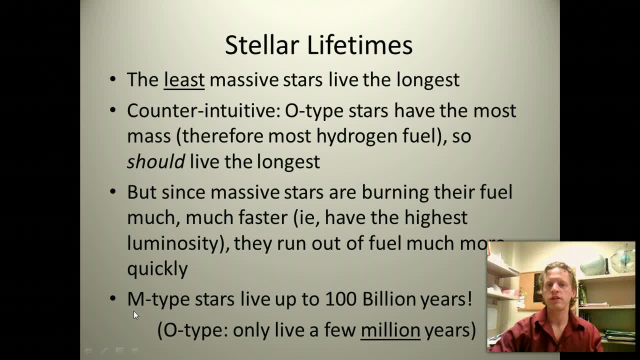 They're not giving off much light at all compared to the other stars. So these are the stars that burn through their fuel so slowly that they can actually live to be over 100 billion years old, Which actually is about 10 times more than the lifetime of the universe right now. 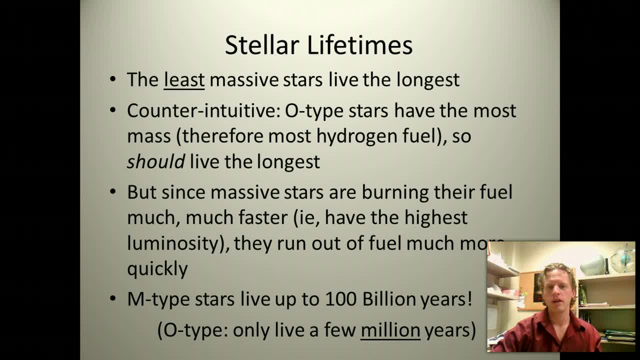 The universe has only been around for about 13.8 billion years or so, Which means that some of these stars that were born, you know, 5,, 10 billion years ago, are going to be around for another 90 billion years. So these are the very, very most longest-lived stars. Some of these stars that were born, Some of these stars that were born right after the universe started, haven't died yet And, for comparison, O-type stars, they can live and die within less than a million years. 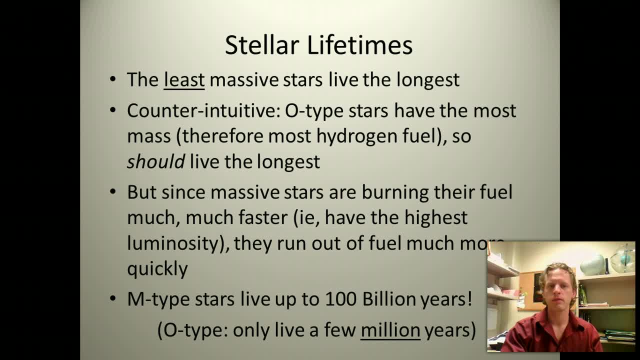 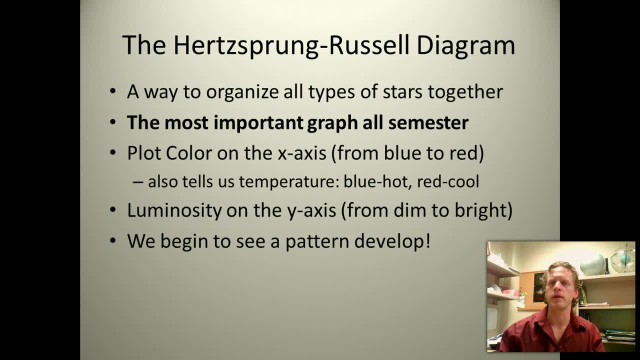 So extremely rapid compared to 100 billion years. Okay, so we can put all of this together. All of these properties, the lifetime, the mass, the size, temperature, color, luminosity, all of that stuff we can put into one diagram. 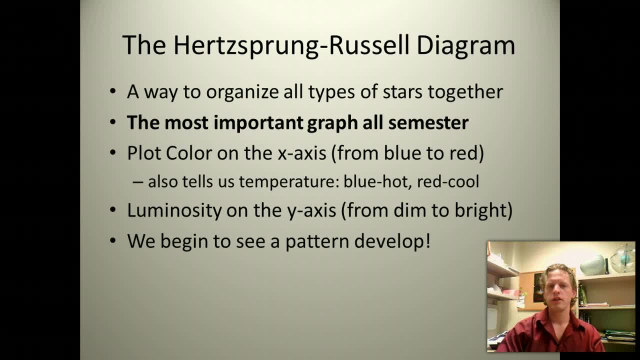 And this is the single most important diagram that you're going to learn all semester, So it's called the Hertzsprung-Russell diagram, or HR diagram for short. Whenever you see HR diagram, it means the Hertzsprung-Russell diagram. 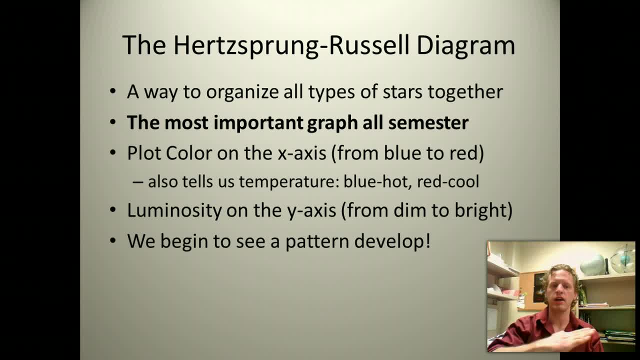 And the point here is that we're going to take the x-axis and we're going to plot out the color of it And, if you remember, the color is actually directly related to the temperature. So the x-axis plots out either- you can think of it as color or temperature. 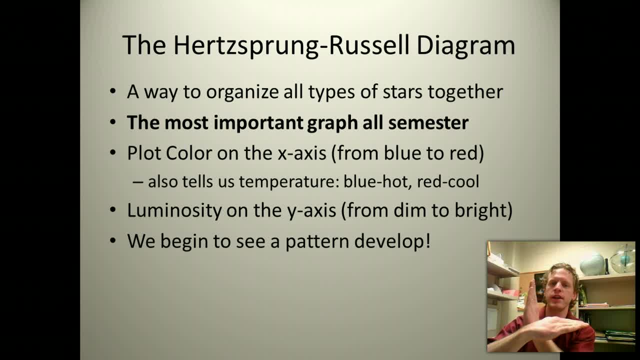 And then on the y-axis we're going to plot out the luminosity, How much light the star is giving off. And the cool thing is, when we do this and we put in all the different types, the O's and the B's and the A's and stuff, we can see a pattern directly developing here. 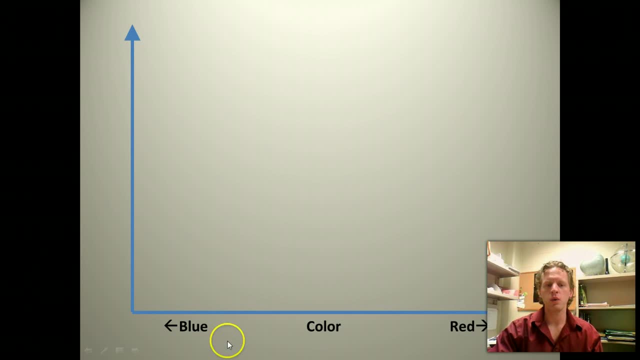 So let's start out. Here's just the axes, Okay, And we start out with putting color here, And the convention is we put the bluish stars on the side and the reddish stars over here, And so, like I said, this relates to the temperature. 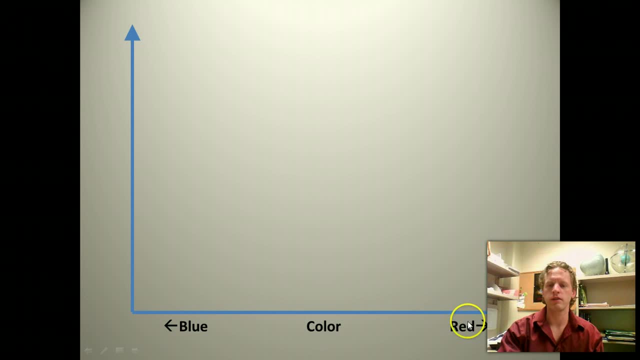 And we know that the blue, the bluer stars have a higher temperature and the redder stars have a lower temperature. So you can also label it like this, if you like: The temperature increasing in this direction And then the y-axis we plot out: luminosity. 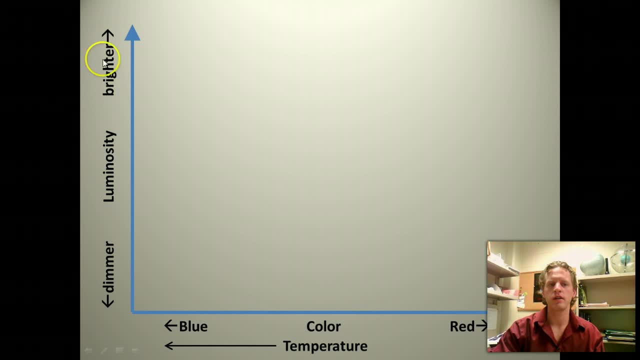 And with luminosity, we're going to plot the brighter stars, or the stars giving off more light to the top, and the stars giving off less light, Or the dimmer stars on the bottom. And so what we're going to do, first of all, we're going to find where we will put the 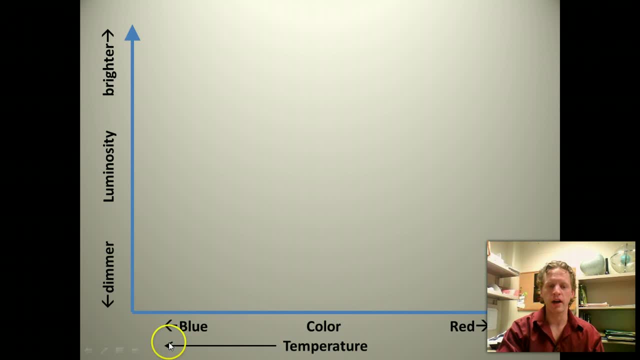 O stars. Now we know, first of all, the O stars are very hot and they look quite blue to us, So they're going to fall on the left side of this diagram here. But we also know they're extremely bright. They have the most luminosity. 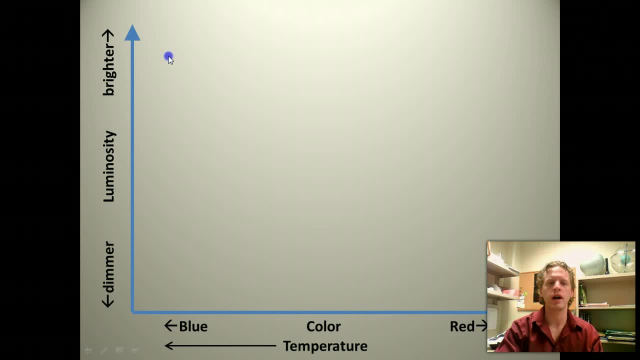 So they're going to fall on the left side of the diagram and they're going to fall all the way at the top. So there's O star. So any stars that are O-type stars are going to fall on the top left of this part of this. 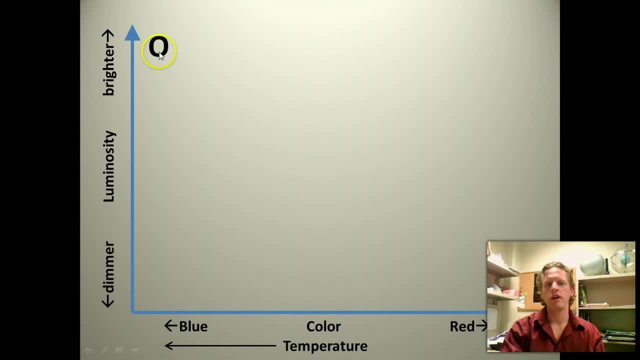 diagram here. Now, if we go to B-type stars, they're a little bit less luminous and a little bit cooler, or a little bit redder, if you will. So the B-type stars are going to be. where's my mouse? there it is. 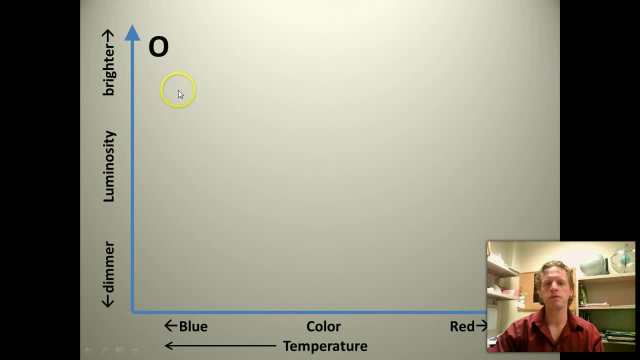 So the B-type stars are a little bit lower and they're also a little bit further in this direction because they're a little bit cooler. So there's the B-type stars. Now, when we go from B to A, an A-type star is just a little bit less luminous than a. 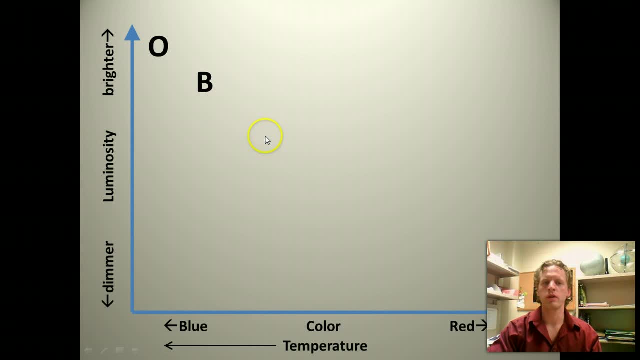 B, It's not giving out quite as much light and it's a little bit cooler yet. So we go down and to the right, And that's where we find our A-type stars. And we can keep on doing this For each type. we go down in luminosity and we go to the right in temperature a little. 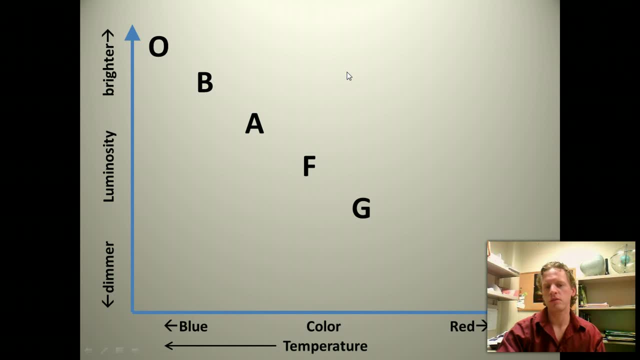 bit cooler each. So there's the F-type stars, there's the G-type stars, there's the K and finally the M. So we see that the M stars lie all the way to the very red part of the spectrum, or they're. 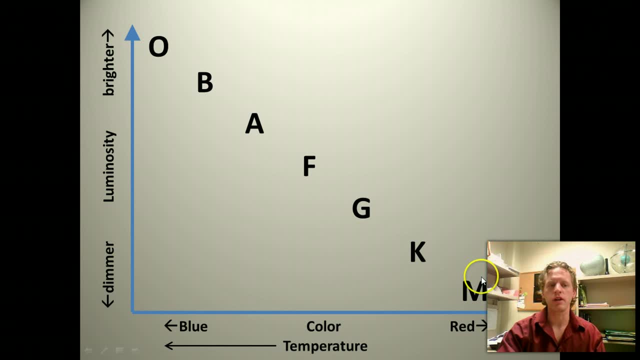 the very coolest stars And they're also the very least luminous on this axis They give up the least amount of light, So they fall at the bottom right. So here's the pattern. We see this nice diagonal line running from very luminous and very hot to very dim, and 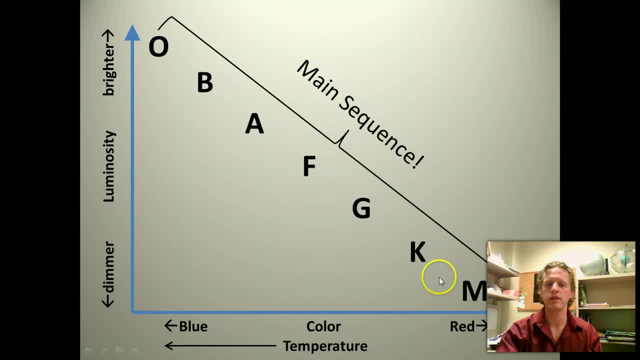 very cool. So this whole thing is- this is why we have the name- the main sequence. It's not a sequence like a set of steps that a star goes through in its lifetime. It's not a time sequence. It's a sequence on this direct diagram. 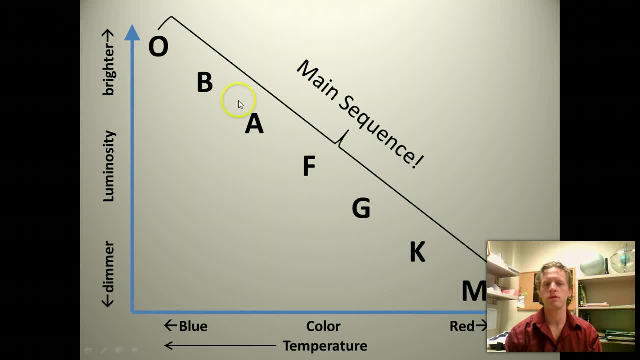 So this is where that name main sequence comes from. It's a sequence of stars going from upper left to lower right on this HRD. So that's the basic idea, That's what the main sequence is here And, like I said, if you can place any of these stars into a category here, so if you know, 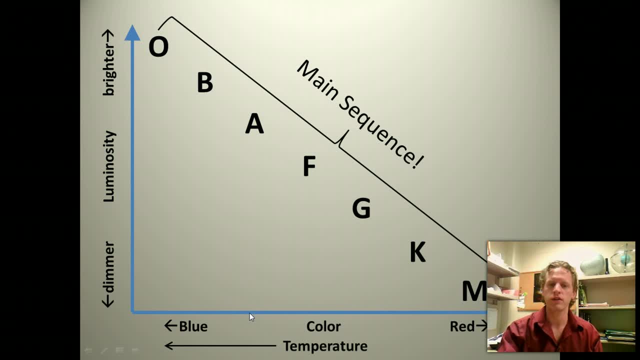 it's an A-type star. you can look down and you can figure out exactly what temperature it must be or exactly what wavelength it's giving off of light. You can also look over here, and if I had these labeled, if there were labels for the luminosity. 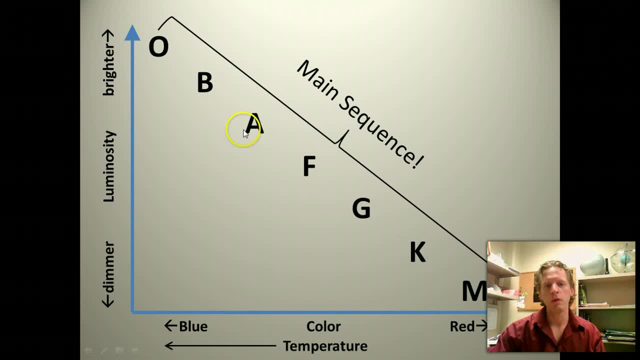 you could tell exactly what the luminosity of the average A star is. And when you know those things, you can figure out the mass. When you know the mass, you can figure out the luminosity. You can use those to figure out the lifetime. 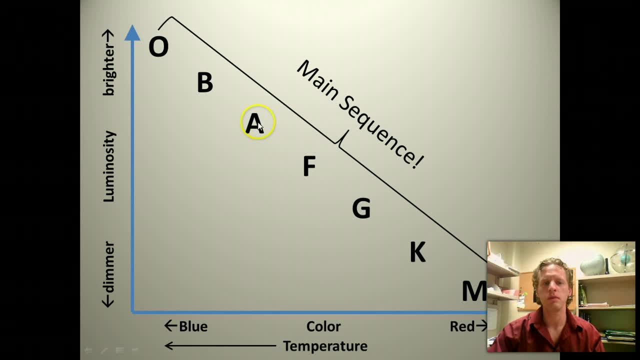 We're not going through this. So once you know even one of those properties, you can basically take an average value of those properties for that class of star and figure everything else there is to know about that star, as long as it's a main sequence star. 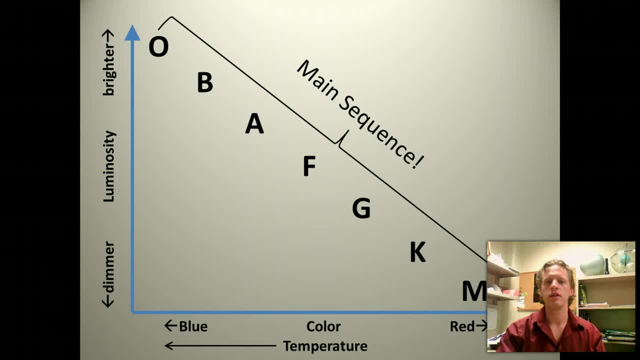 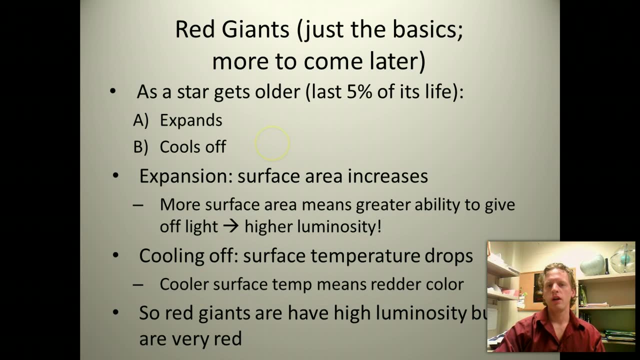 That's actually a really important point. If it's not a main sequence star, this stops working. So let's talk about some of those non-main sequence stars, So red giants, for example. What a red giant is? it's a star at the very end of its life. 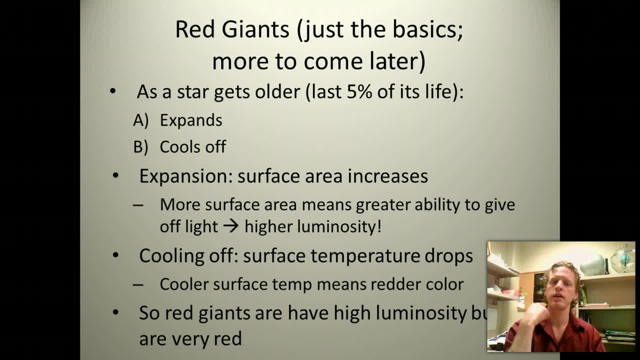 In the last 5% or so of its life, right before it's about to die. what happens is: A- it gets bigger, so the giant part of it, and B- it cools off, So first of all the expansion part of it. as it gets bigger, it has way more surface. 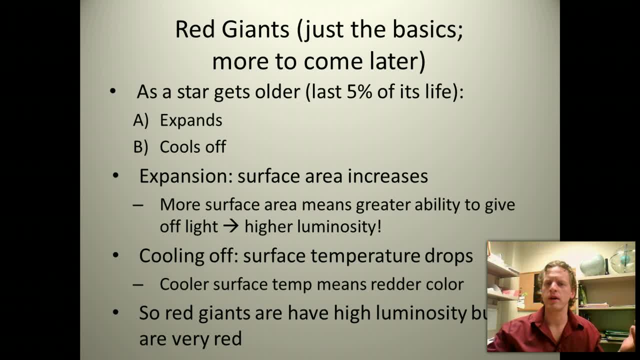 area to give off light. The way I compare this is if you have, let's say, a billboard that has 10 LED lights by 10 LED lights, so you have 100 LED lights there. you're giving off some amount of light. 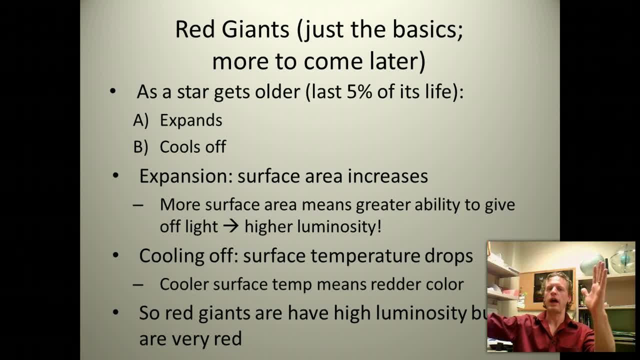 Let's say you make that board, you stretch it out, so there's 100 LED lights this way and 100 LED lights that way. Now, all of a sudden, you have 10,000 LED lights. The brightness of each of those lights hasn't changed, but the overall amount of light given. 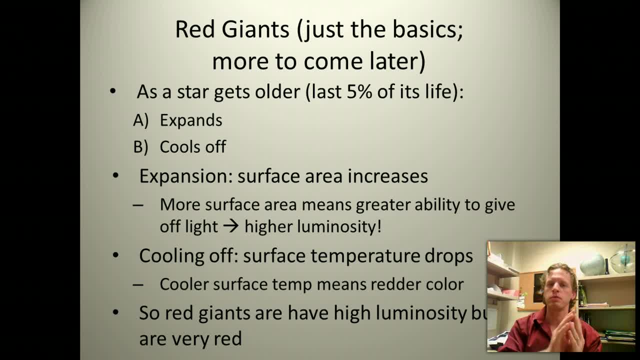 off by that really big board is a factor of 100 bigger than it was before, just because you've increased the area of that sign. And that's basically exactly what's happening with these red giants: You make them much bigger by a factor of 100, or 10,000, or even a million times bigger. 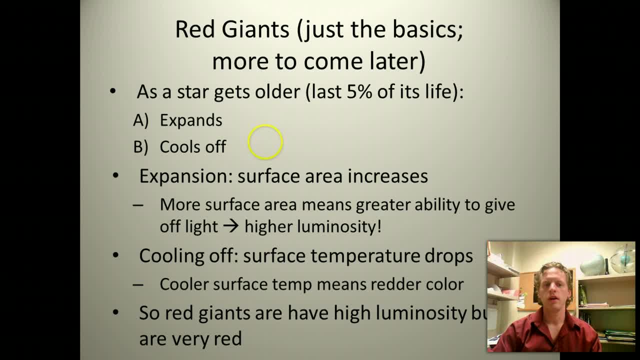 and you end up giving off way way more light. So that's a big difference. It gives off more light than the star used to. So as the star expands, its surface area increases and it gives off more light, so it's more. 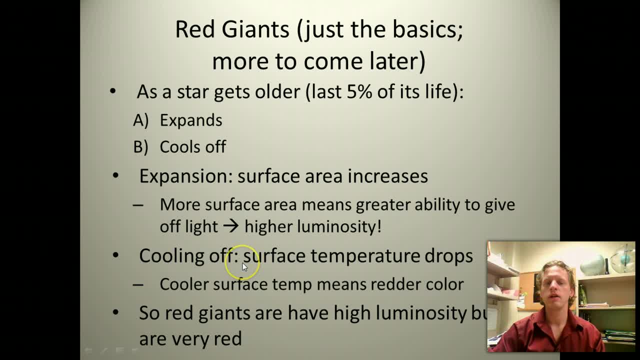 luminous. Now, as it cools off, something else happens too. We know that hot things give off blue light and cold things give off red light. So as the star expands and cools off, it also becomes redder, and that's hence the name. 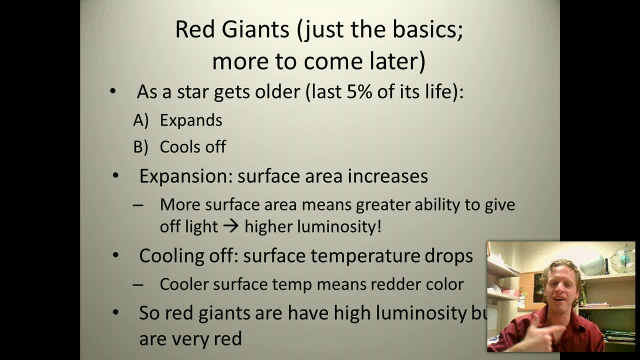 Red because it's cooler and giant because it's giant. So that's what a red giant is: It's a star at the end of its life, which it's expanded and it's cooled off. Now it looks redder to us. 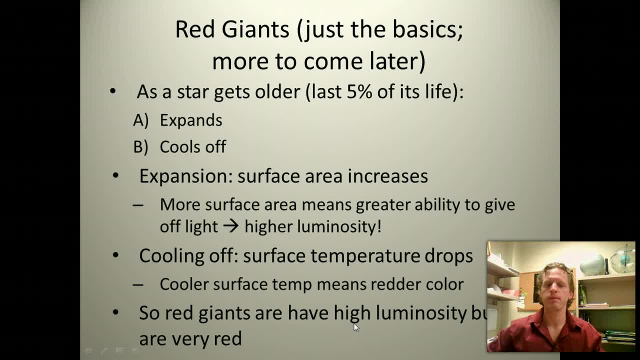 So red giants have a very high luminosity because they're so big and they look significantly more red than they used to back when they were in a main sequence phase of their life. So here's where the red giants are going to be. We have the main sequence again. 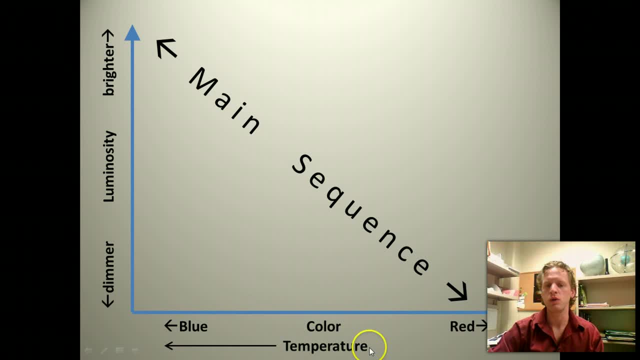 And let's take a red giant. We know the red giants are relatively cool or they look red. So we look to where the red is here. and we know red giants because they're also extremely large, huge amount of light, So they're also quite luminous. So a red giant is going to be all. 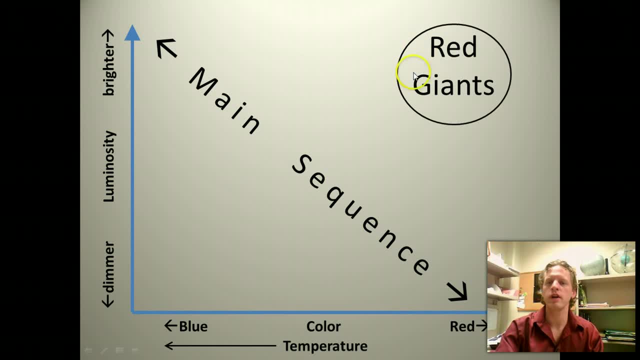 the way to the right and then all the way up. So this is the red giant reaching the spectrum or of the diagram. By the way, in your book you're also going to see some more stuff called supergiants and superbluegiants and blah, blah, blah. I'm just generically. 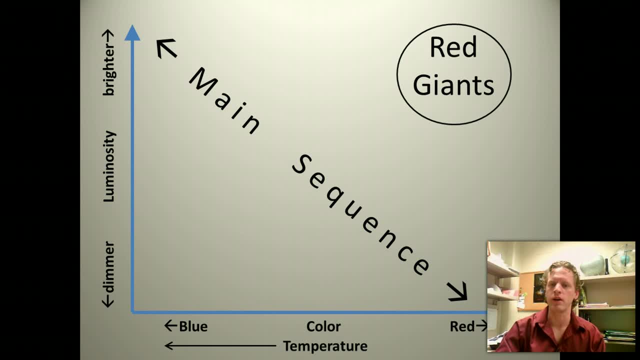 grouping all of this into the red giant area of the diagram. here, When we talk more about the death of stars, we'll see what the difference is between a supergiant and a red giant, But for all purposes it's effectively the same thing. So that's where the red giants are. 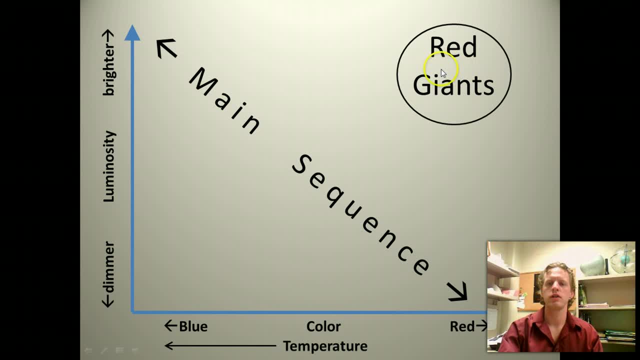 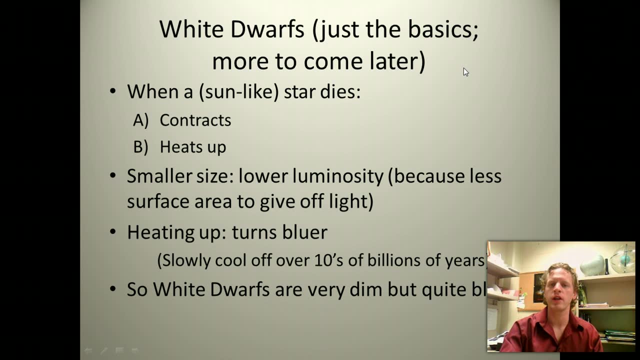 again, because they're bigger, so they're more luminous and they're cooler, so they look redder. Now one more thing: The textbook mentions something called white dwarfs, And again we'll get to this later in the semester, but a white dwarf is actually even after. 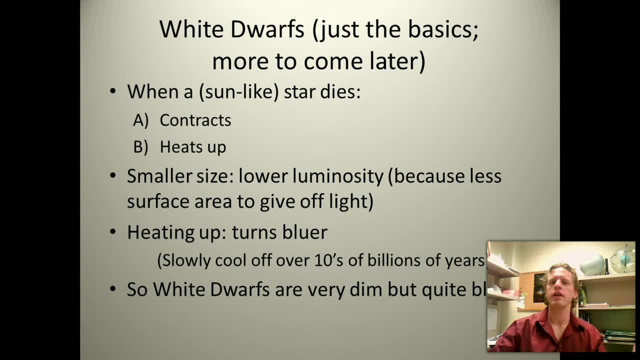 that red giant part of the lifetime. after that star has finally given off its last gasps, it contracts. It actually becomes about the size of the Earth. So you take a star and you take a star like our sun. it expands out to include all of the orbit of Mercury. 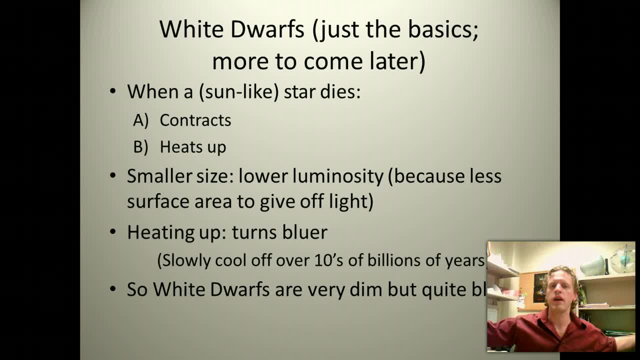 Venus, Earth, maybe even Mars in its red giant phase, and then it contracts to be as small as the Earth, And that's what a white dwarf is. As it contracts, it also heats up to very high temperatures. So because it's getting smaller, the surface area is increasing. 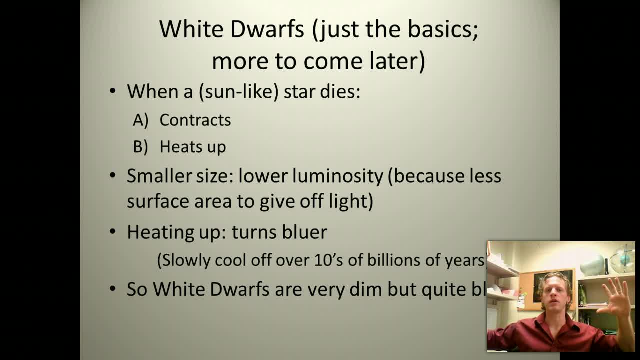 So you're taking that 10,000 LED light bulb billboard and you're decreasing it to just a billboard with maybe three or four lights. Those lights might be giving off a little bit more light. It gets a little bit hotter Each of those individual lights are giving. 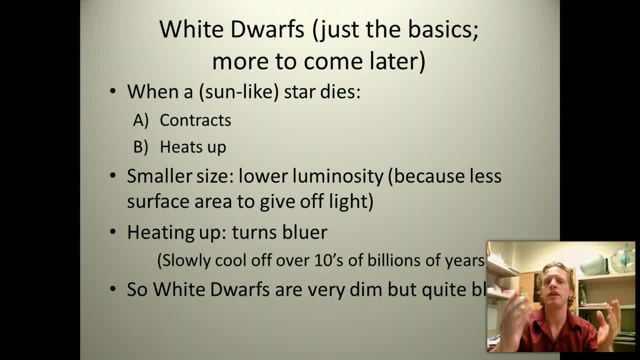 off a little bit more light than they might have before, But the overall amount of light is much reduced compared to that big giant billboard that it just was. The analogies are kind of stopping to work here, but the point is, when you decrease the size, the luminosity also decreases. So as a star becomes smaller it loses its luminosity, but it also gets hotter. It's taking all that heat and compressing it and contracting all that heat into a very small ball, so it actually heats up. 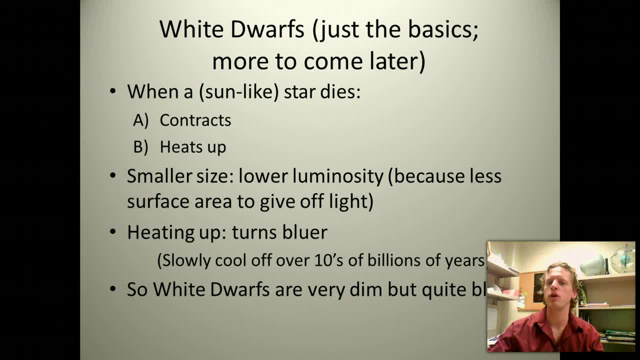 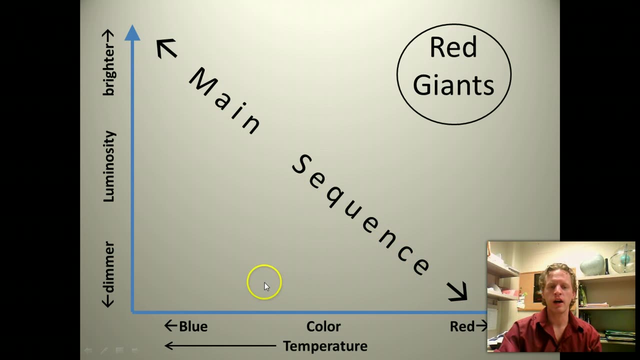 And very slowly over the course of tens of billions of years it will very slowly evaporate that heat away. But a white dwarf shortly after it forms is very small, so not very luminous, but extremely hot. So when we look here we take the main sequence and now we go to the very hot end of it, the 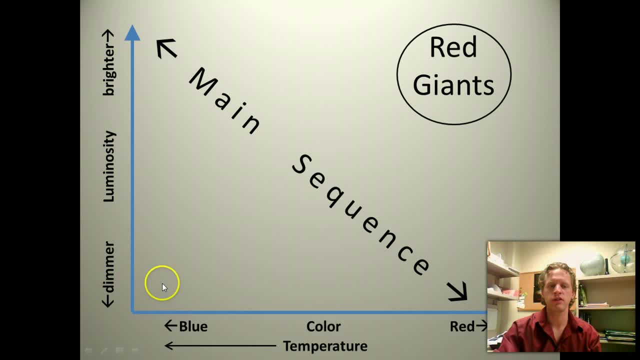 very blue end and the low luminosity because its surface area isn't very large And that's where the white dwarfs are. So this is the overall picture that you should be incredibly familiar with. This is, again, the most important picture, the most important diagram. we'll cover this. 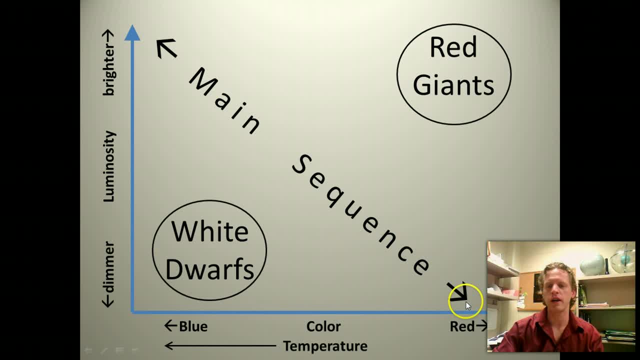 semester. The main sequence extends from low luminosity red stars- the M-type stars- to high luminosity hot blue stars, the O-type stars. The red giants are up there because they're very large, so a lot of surface area to give. 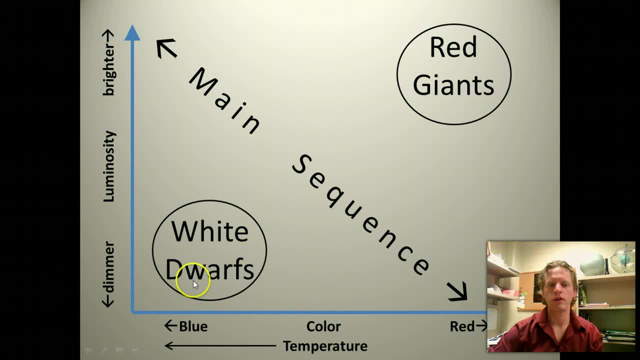 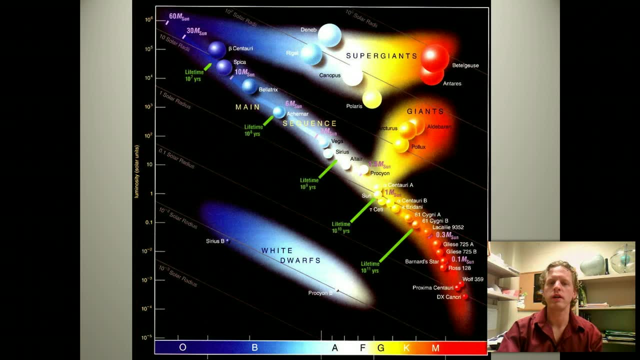 off a whole lot of light, but very cool. And the white dwarfs are down here because they're very small, so not much surface area to give off light, but incredibly hot. And just to show you what a real diagram would look like: 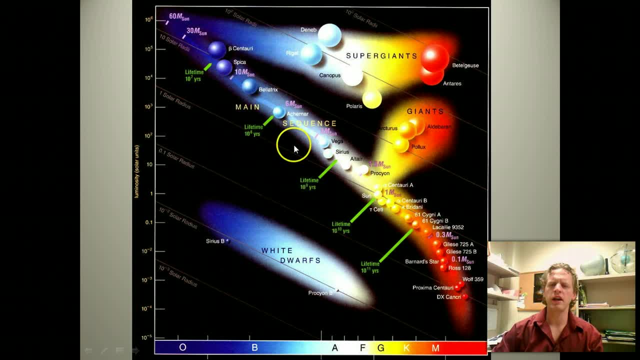 I've taken some artistic shortcuts there, but it gets a little more complicated And you see there's a slightly separate region for the giants and the super giants. But again, it's typically to the right and above the main sequence And down here the white dwarfs. 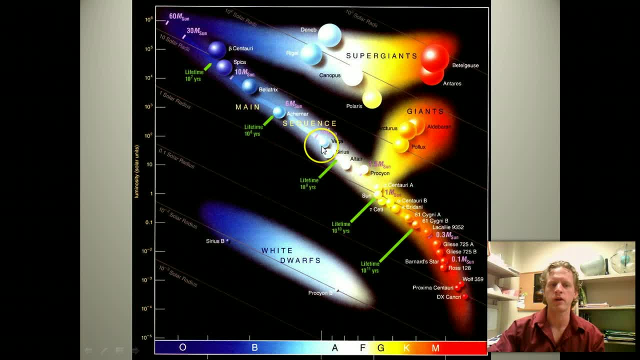 Now it's labeled many actual individual stars here, so it's kind of cool. Look this up in your textbook and you can see each of the individual stars. But, by the way, so the sun is a G-type star. It's about halfway in between the O's and the M's. 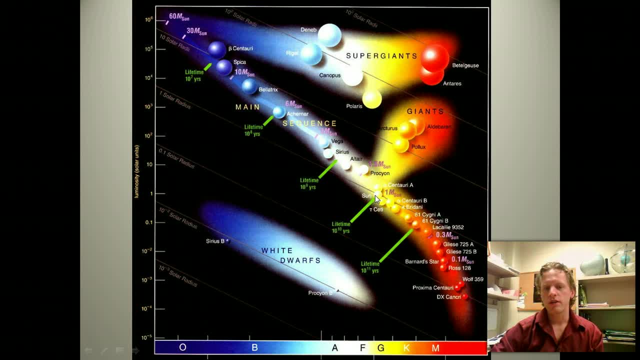 And the sun here. you can see it right there. So the Sun falls in the G-type spectrum and it has luminosity, you know, kind of high, not too high. So the Sun is actually kind of a Goldilocks-type star. 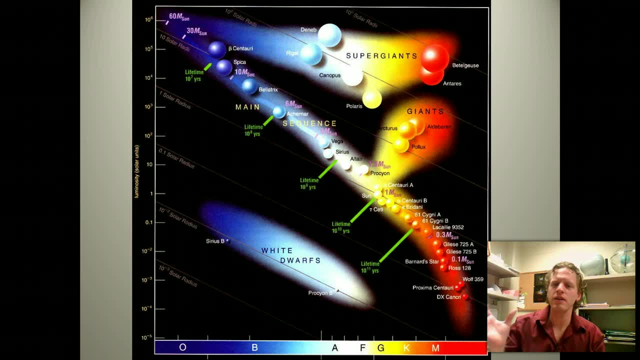 It's not too big, it's not too small, it's not too hot, it's not too cold. It's kind of right about in the middle of all of these properties, which is convenient for us because it seems to be the most likely type of star that you can form life around. 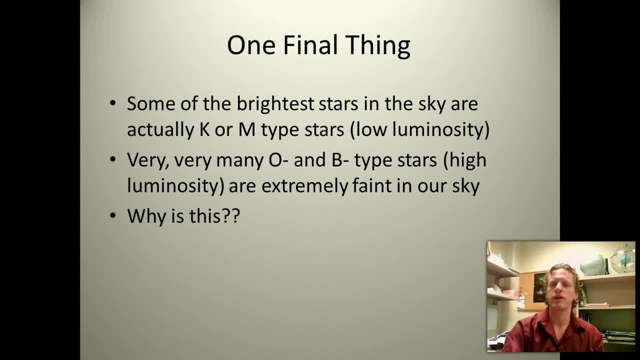 so it works out Alright. so one final thing here. The book spends quite a bit of time talking about the distance-luminosity-apparent-brightness relationship, and so it gets a little confusing. The book makes it more confusing than it really should be. 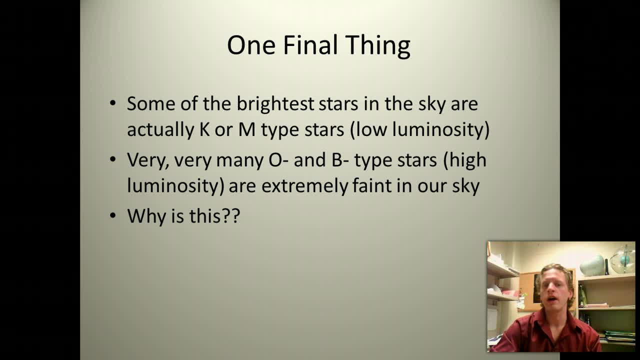 So the idea here is that some of the very brightest stars we can see in our sky are actually K- and M-type stars, or maybe G-type stars, like our Sun. They're not really that luminous, but they're very bright to us. 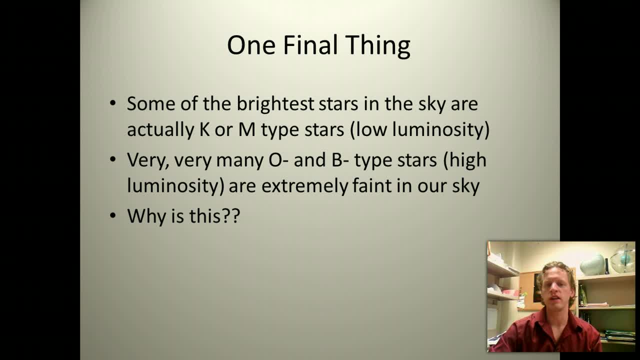 And also, on the other hand, some of the very most massive stars we can see in the entire sky are some of the dimmest stars that we see as well. It's not because They're incredibly massive and it's not because they're very high luminosity. It's due to a different reason. So the reason that you can have a low luminosity star look very bright and a high luminosity star look very dim is the distance. If you take something that's really dim but put it right in front of your eye, it's going. 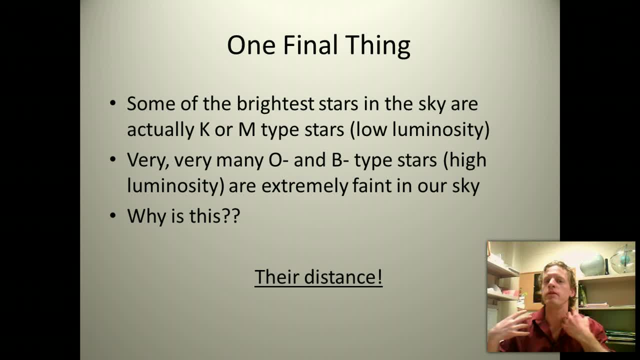 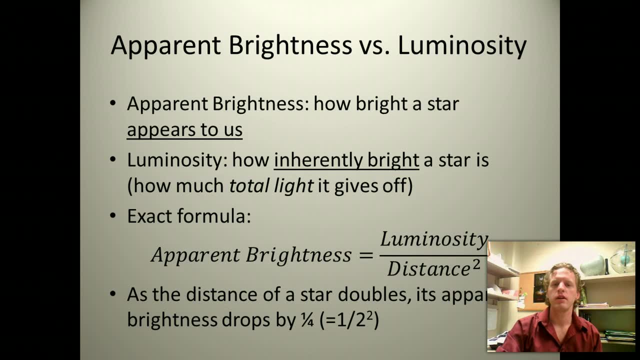 to look really bright to you, But if you take something that's incredibly bright and move it onto the other side of the galaxy, you probably can't even see it, And that's basically what's going on. The term for this is apparent brightness. 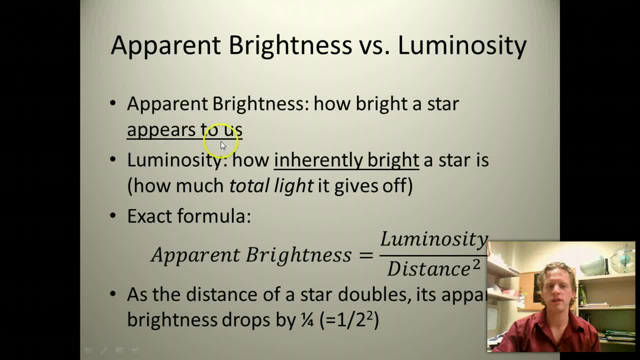 So the apparent brightness refers to how bright the star looks to us, How bright it appears to us, hence the name apparent. If a star looks really bright to us, it might mean that either it has a very high luminosity or it might mean that it's just really close to us. 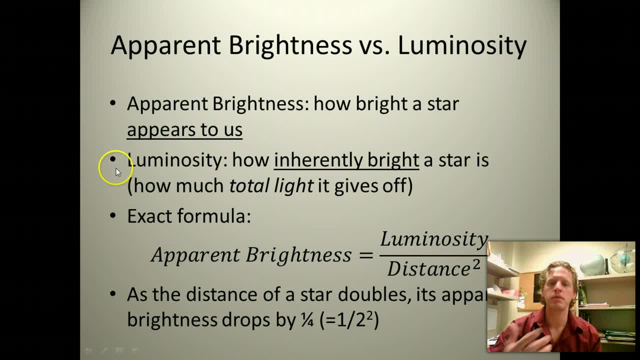 So compare that to the star's luminosity. The luminosity is an inherent property of the star. It's how much total light it gives off, regardless of how close or how far it is to us. So everyone in the entire universe will agree on a star's luminosity. 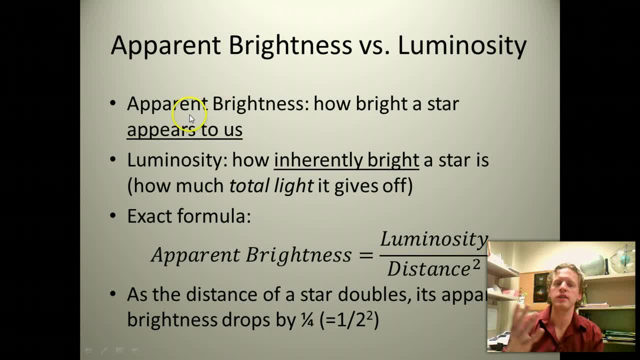 But not everyone will agree on a star's apparent brightness. The people very close to that star will say it's bright. But not everyone will agree on a star's apparent brightness. If it's bright, the people very far from that star will say it's very dim. 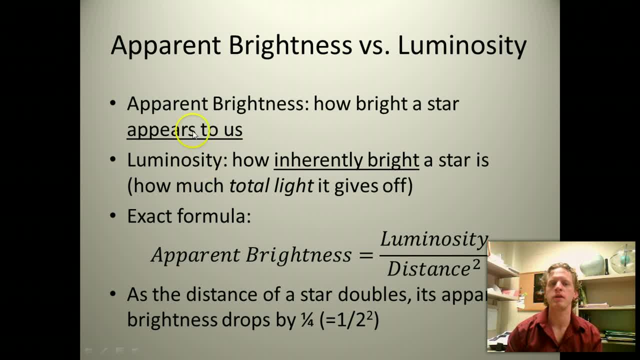 So the luminosity is an inherent property- the total amount of light, whereas the apparent brightness depends very much on how close to that star we are. Now the exact formula for this: the brightness depends on the luminosity. You double the luminosity, it appears twice as bright to us. 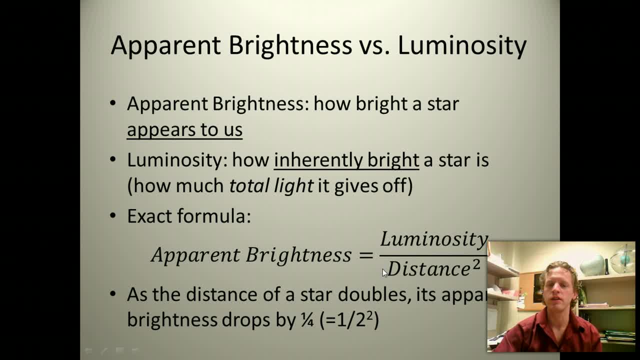 But it's inversely related to the distance squared. So what that means is if you double the distance, the star looks four times dimmer. If you triple the distance, The star looks nine times dimmer- One over three squared, or one over nine. 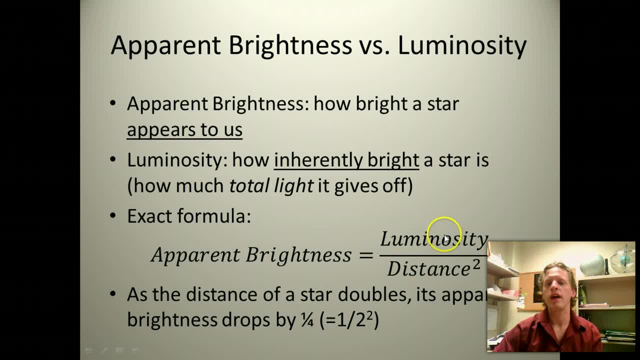 So it's actually the distance plays more of a role than the luminosity. That's why you can have extremely luminous stars that look really dim, because the distance is very, very much related to the apparent brightness of the star. So, again, we're not going to be doing direct calculations, but that's the basic idea. 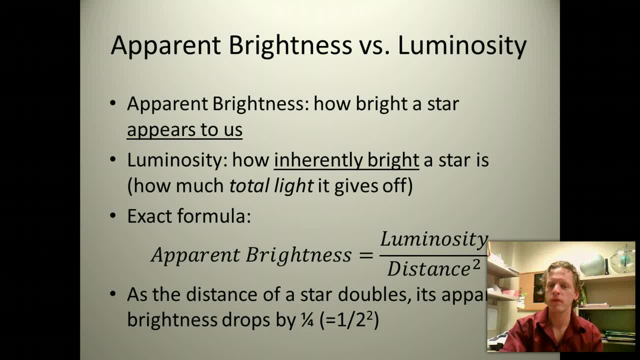 And there's some rules that we can follow to derive this, but I don't want to get into that. I don't want to bore you here, All right. So just to wrap all this stuff up here Again, make sure that you're using a calculator. 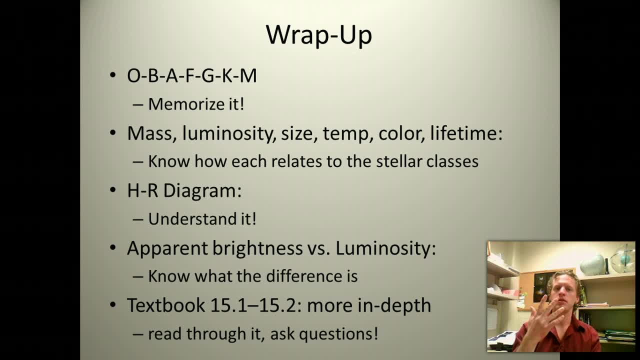 You're going to need a calculator. Make sure you memorize the O, B, A, F, G, K, M scheme And this. you're going to need to know this definitively. You need to know exactly what order all those are. 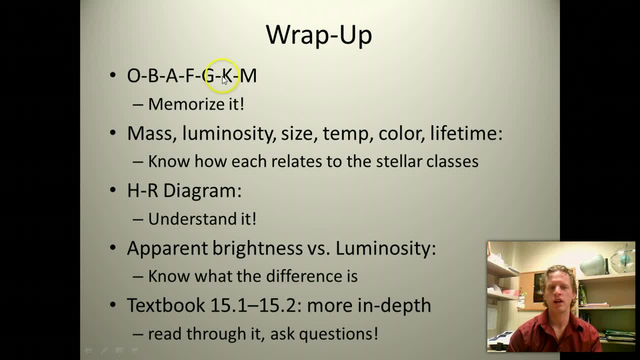 You should also know how the mass varies as you go down that end or go down that line. You should know how the luminosity goes from the O to the M, how the size, how the temperature, the color and the lifetime are all related to those characteristics. 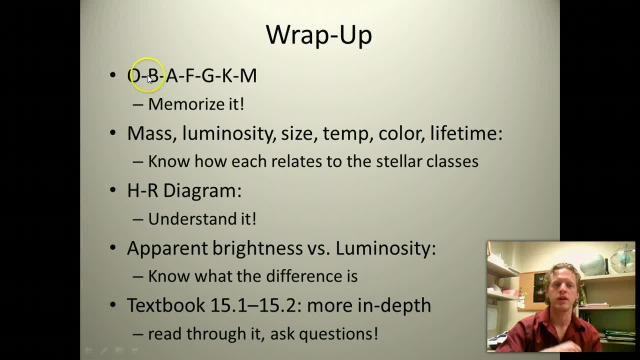 So I can tell you right now. there will be questions on the exam saying which is more luminous, a B type or an F type, Or which has a redder color, a G type, or which has, maybe which is redder, an M or. 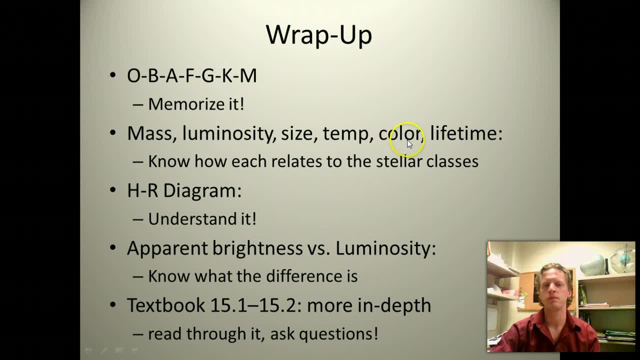 a B star. That gets a little difficult to quantize, but the point is you should know how each of those varies as you go up or down the line And you should definitely understand what the HR diagram is about. If I tell you you have a really luminous but a pretty cool star, you should tell me. 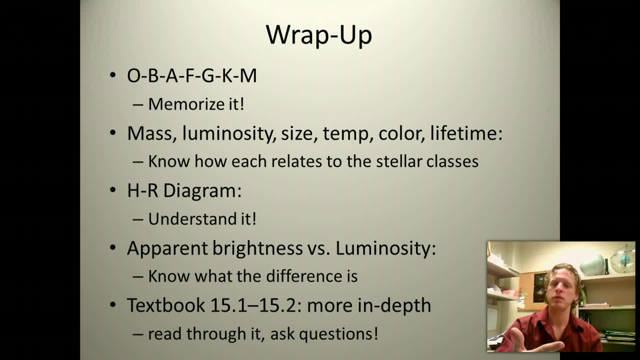 where that goes. If I tell you that you have a star that's medium luminosity but extremely luminous, but extremely hot, you should tell me where that goes and so on. So make sure you understand how that works And you should at least understand the basic idea: the difference between the brightness. 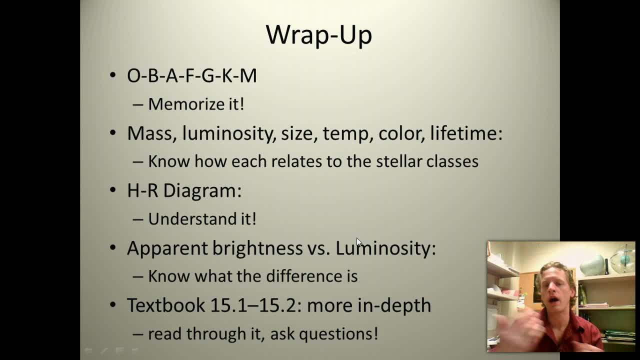 the apparent brightness and the luminosity, Know what the differences between those are and know how the apparent brightness depends on the luminosity and the distance. Again, you're not going to need to solve mathematical problems, but at least understand the basic idea behind it. 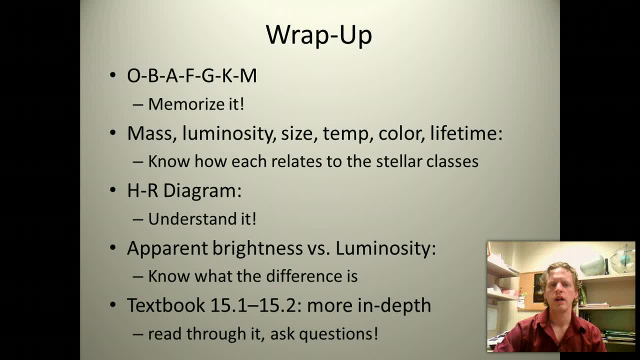 And then, finally, do please read through 15.1 and 15.2 in your textbook. This goes into quite a bit more detail than what I typically would in class, So I'm going to read through 15.1 and 15.2 in your textbook. 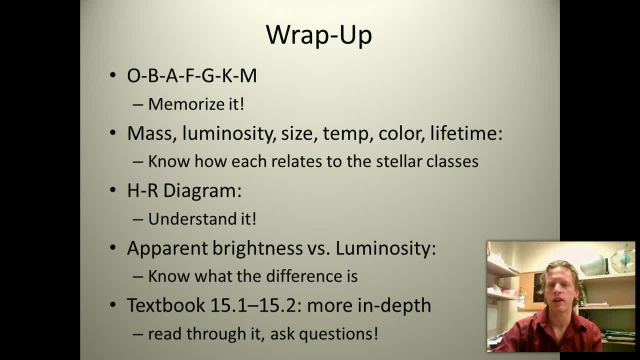 This goes into quite a bit more detail than what I typically would in class, But hopefully you're actually understanding a lot of this as you go through. If you do have any questions, by all means please contact me. I'll be happy to do my best to put you on the right track. 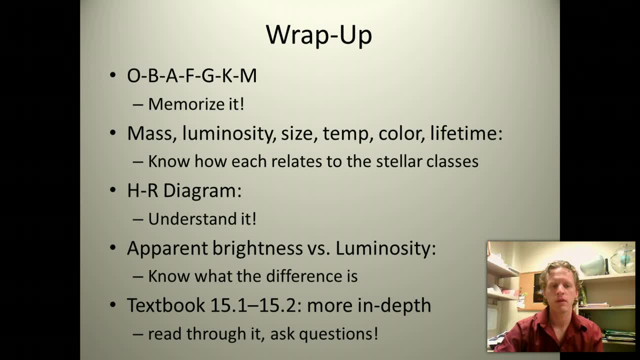 And I know this is a little bit more difficult stuff. So if you are understanding all this, good job. If you're not, again please feel free to ask. But all right, that's about it. Let me know if you have any questions about this again. Bye.